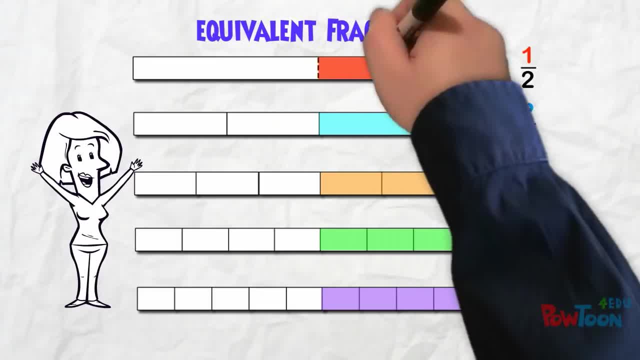 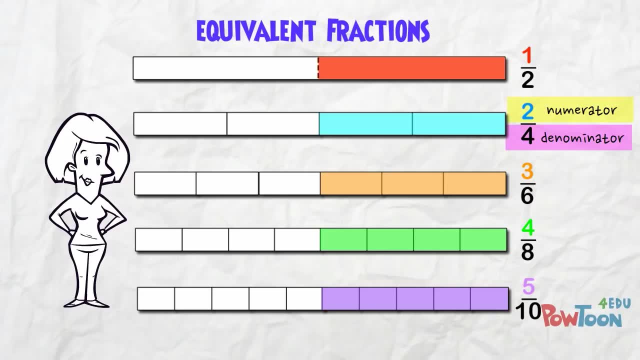 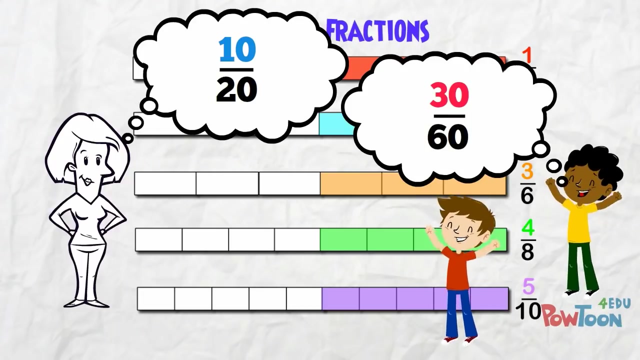 You can see, these are all equivalent fractions. Notice that the denominator is 2 times its numerator for all these equivalent fractions of one half, And you could easily think of some more like this without using fraction strips. I want you to take a note. 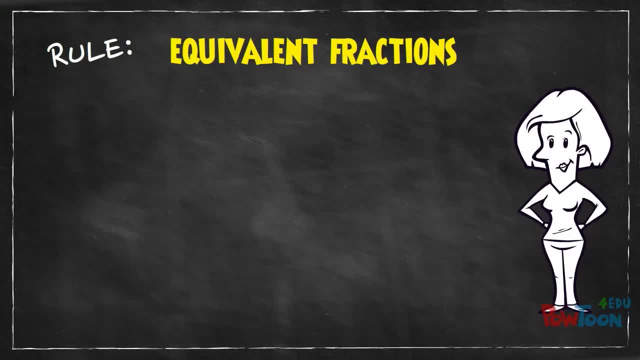 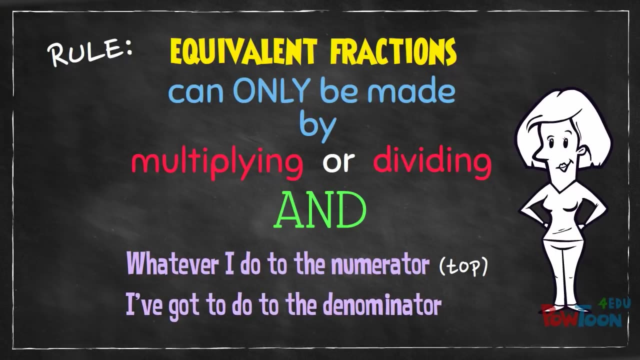 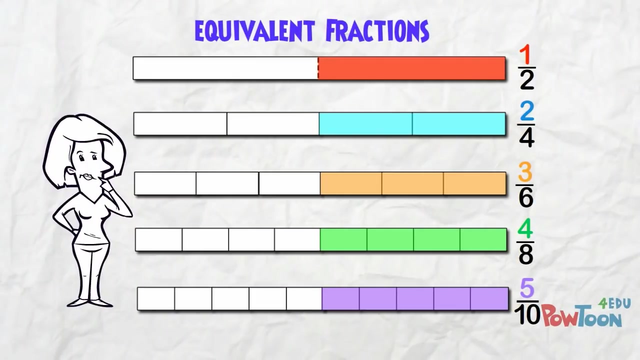 The rule is by multiplying or dividing, And whatever I do to the numerator- the top number, I've got to do to the denominator, the bottom number. Now let's go back. These equivalent fractions of one half have bigger numbers, But we can see they all have the same size value. 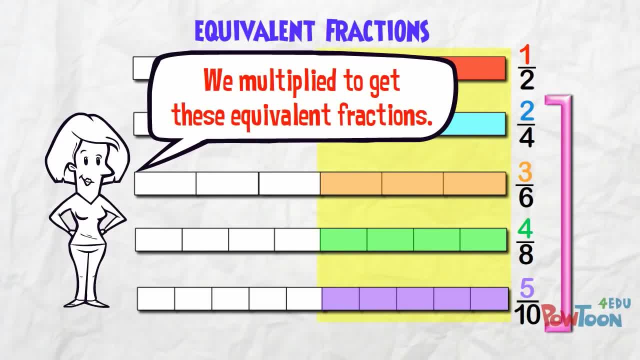 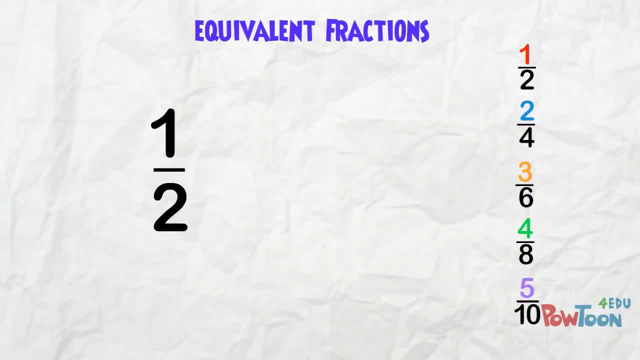 So we multiplied to get these equivalent fractions. Now let's think about that without the fraction strips. Here's one half. What do I multiply the numerator and the denominator by to get this equivalent fraction? I used a factor of 2 to make this equivalent fraction. 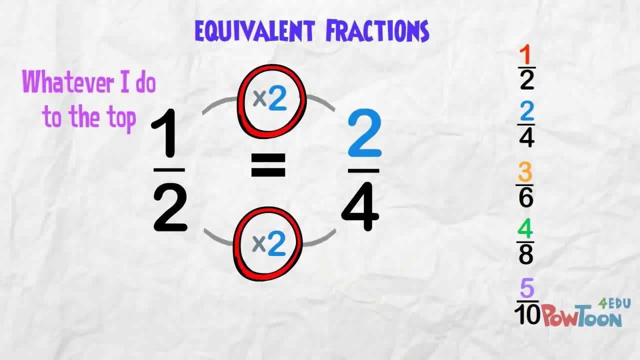 You can see, whatever I do to the top, I've got to do to the bottom. So if I use a factor of 3, I get this equivalent fraction. A factor of 4 gets me this equivalent fraction, And when I use 5, I get this equivalent fraction. 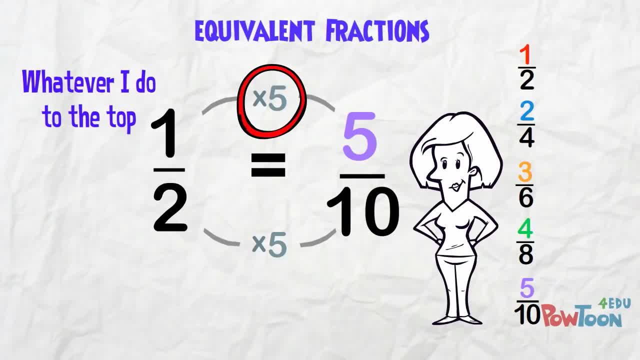 You can see it in action here: Whatever I do to the top, I've got to do to the bottom. That's easy enough, isn't it Ok, then? so let's do some practice to make it stick before you hit the worksheet. 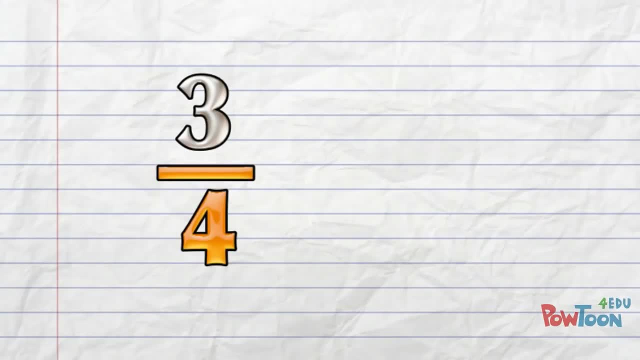 3 over 4. 3 quarters, 3 fourths. What if I make an equivalent fraction using a factor of 2?? Whatever I do to the top, I've got to do to the bottom. 3 times 2 is 6 over. 4 times 2 is 8.